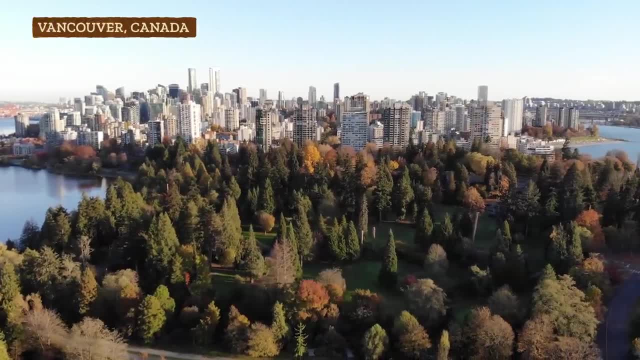 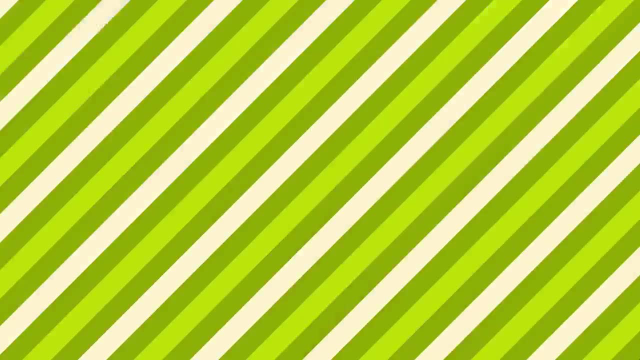 Environmental planning is part of sustainable development, which can mean everything from using natural resources in a way that protects the environment to helping cities grow in ways that can be sustained for generations to come. As environmental planners, this means we focus on creating designs that use natural resources. 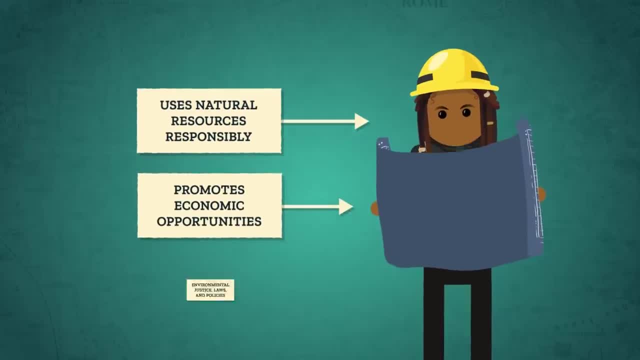 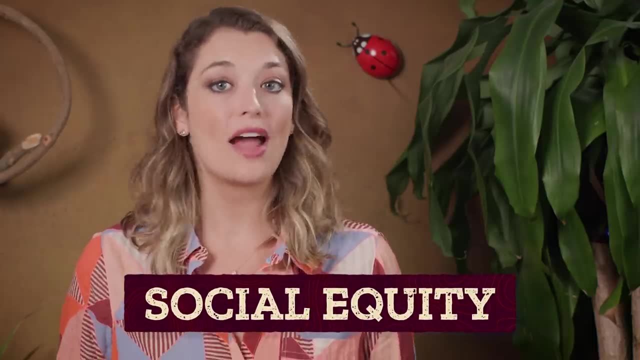 responsibly. We work on how to promote economic opportunities and environmental justice, which is when everyone is involved in environmental laws and policies. We also work on social equity, which is where everyone has just and fair access to things like housing and jobs that pay enough to cover basic needs. 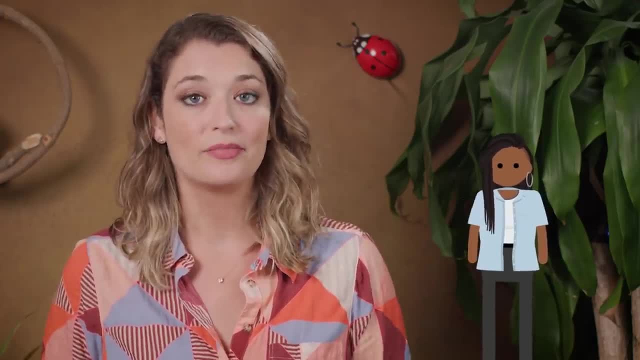 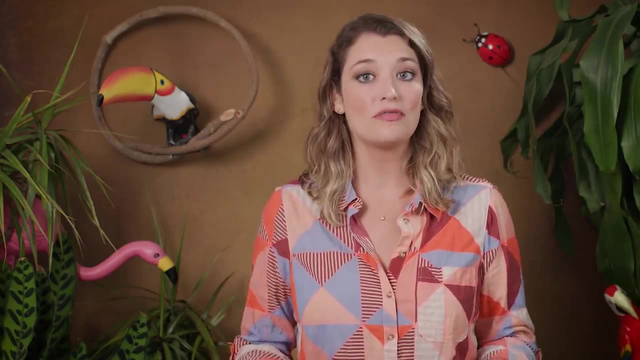 Borrowing a phrase from business. this goal is sustainable And in the end, what's sustainable is the quadruple bottom line: Positive results for people, planet, profits and community. But sustainable development can be a contradiction. What's good for the environment and what's good for the economy don't always match. 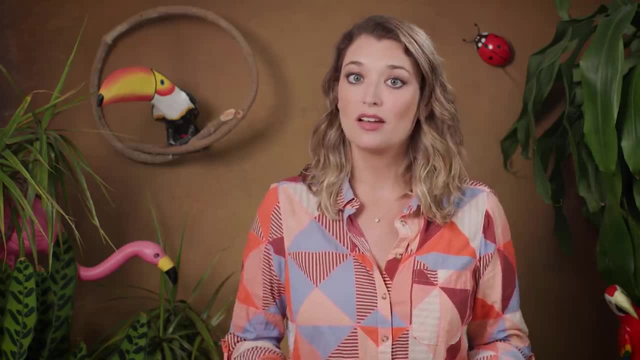 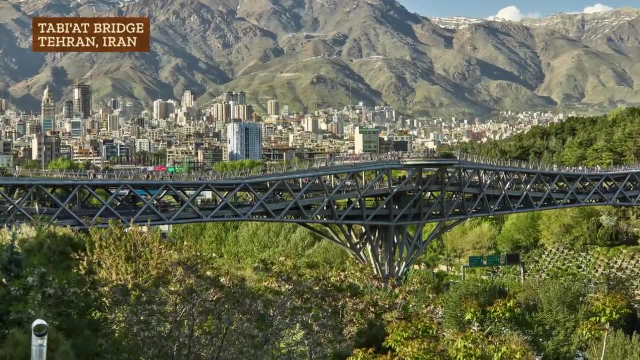 up. So whenever we're trying to sustain or conserve something, a key question to ask is: what are we really trying to conserve? For instance, we might focus on conserving the environment and limiting our use of natural resources, So urban planners will use a host of models and planning tools to help create relationships. 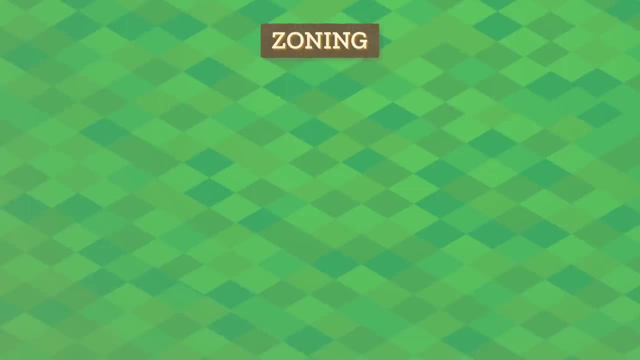 within the city that preserve and use sustainable development. So, what's sustainable? Well, what's sustainable, Well, what's sustainable? Well, what's sustainable. What's sustainable, Well, what's sustainable? open space, Like zoning or designating where different land uses can take place. 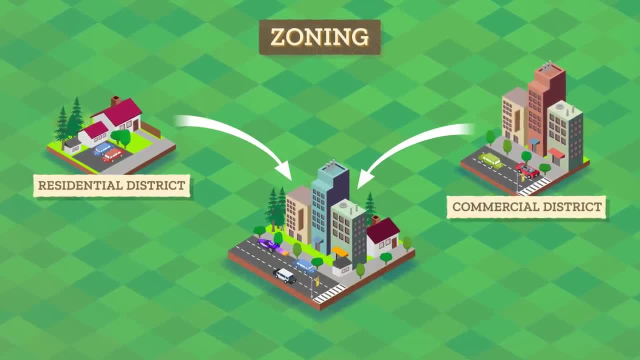 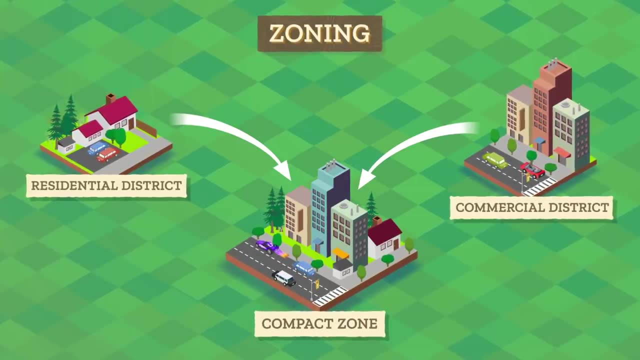 Residential zone. areas of cities can be rezoned or redesignated to create walkable neighborhoods with mixed housing and shops, rather than just one or the other. This creates compact zones where people want to live, work and play, which reduces the need for people to drive across the region. 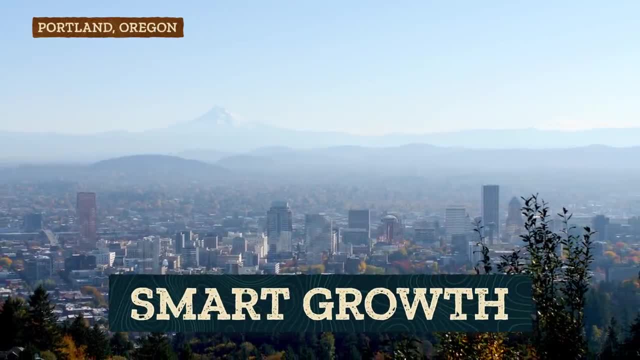 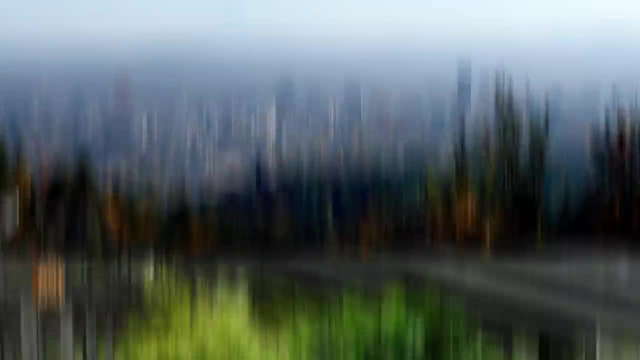 Zoning and other tools are often part of smart growth planning, which tries to control and direct the movement of sprawl or places on the outskirts of cities, like suburbs and edge cities, expanding into open, undeveloped land. In our planning we can also use ecological design, which is an effort to build buildings. 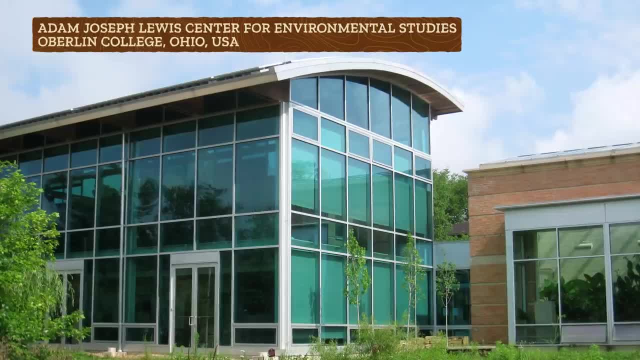 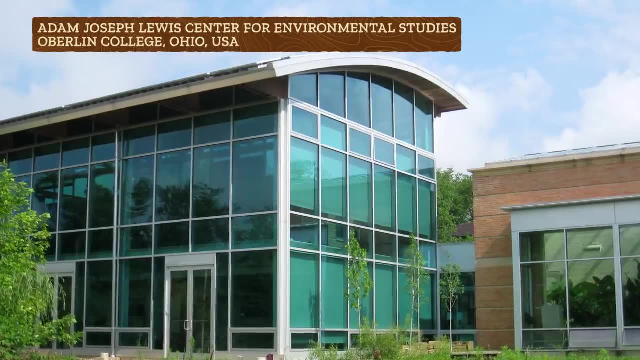 – and even whole cities – to mimic nature, And buildings that are designed like living machines or that emphasize passive solar design. elements that use the sun for heating and cooling are just the beginning. Ecological design is a key place where physical and human geography mix, but, as we've learned, 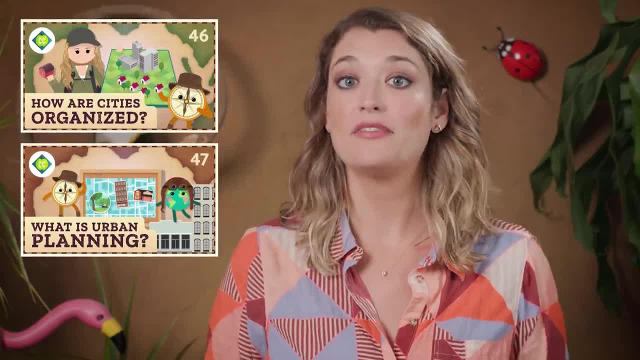 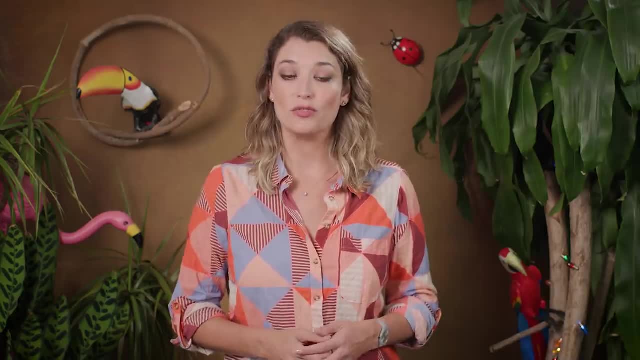 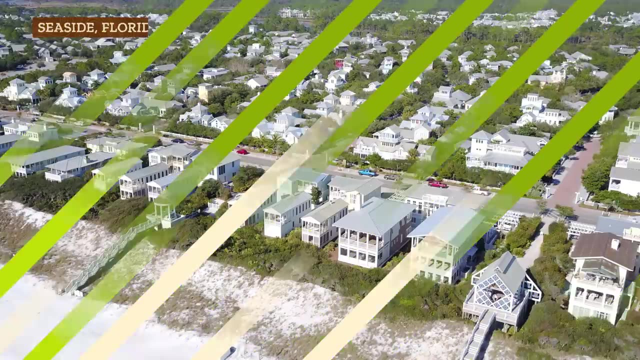 in previous episodes. cities encode a lot about our ways of life and cultures within the design and architecture of their buildings, And we can conserve that too. But no matter what we're trying to conserve, we're going to create tension For one. urban planning is about relationships, so it's rarely a neutral act. 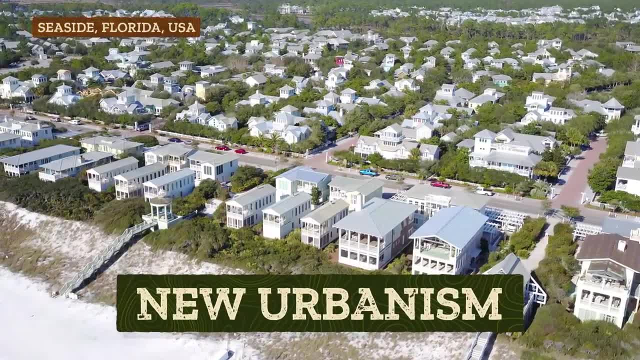 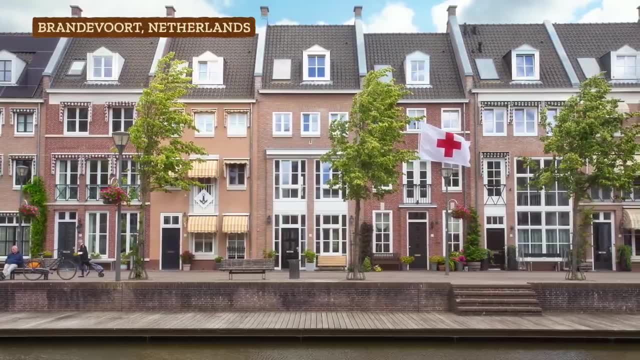 One approach to sustainable neighborhoods includes new urbanism, which is like smart growth, but usually just at the neighborhood scale. It often creates areas people are drawn to, which can then cause gentrification. Gentrification is when the value of land and rent increase in lower-income areas from a 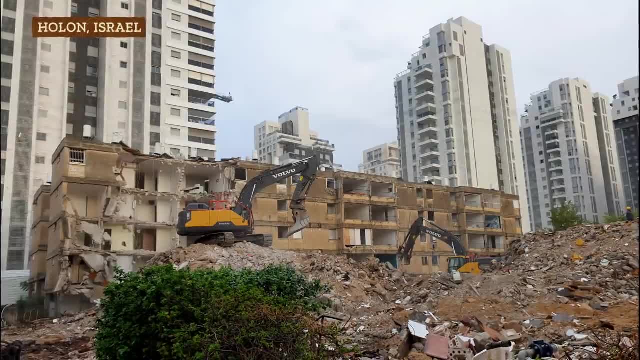 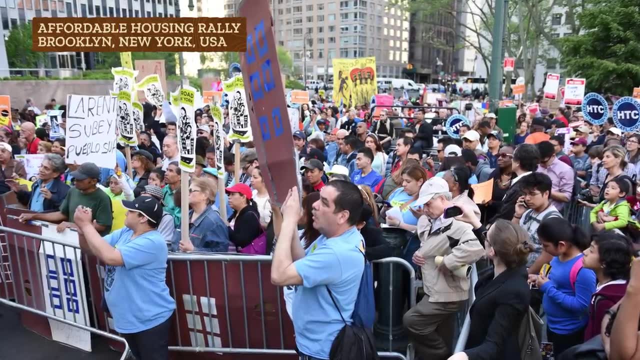 new influx of investment. This growth becomes problematic when urban planning becomes a part of the urban planning process. It's when people aren't treated equitably, as we learned when talking about redlining and urban renewal, If cities don't plan ways to increase economic opportunities for lower-income residents. 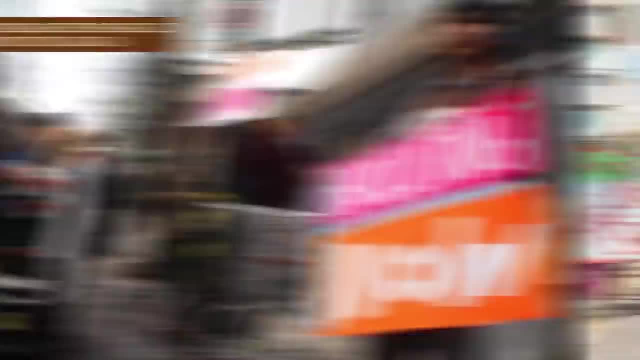 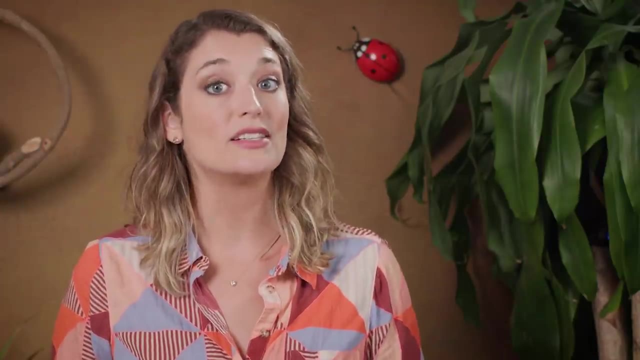 or protect low-income housing. people can be priced out of their neighborhood or city because they can no longer afford the rent. There's no one solution or easy answer to this problem, But we can at least start by staying focused on the people involved and the history of 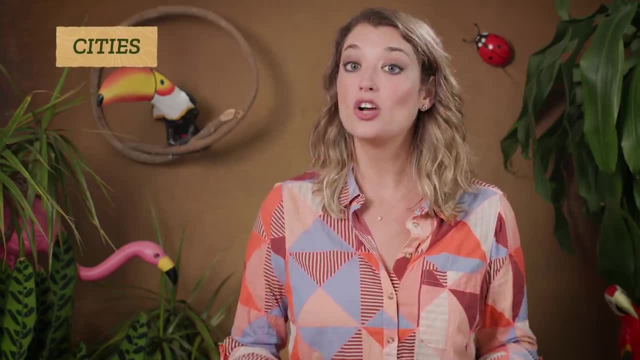 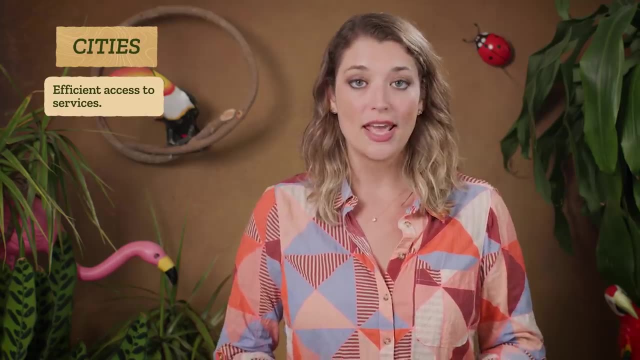 the area, keeping equity in mind. In cities we've also got large concentrations of people, and that allows for efficient access to services like healthcare and the like. Public health care, public transportation and education, And things like electricity or internet access are cheaper. 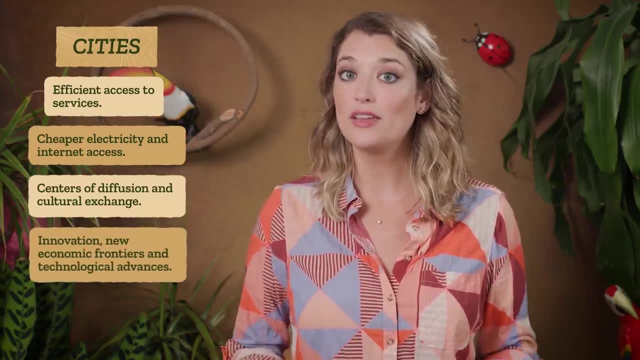 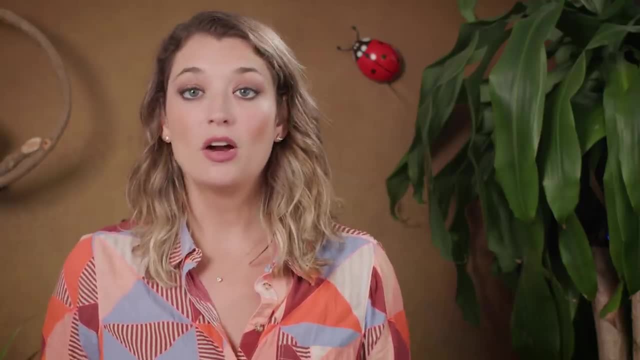 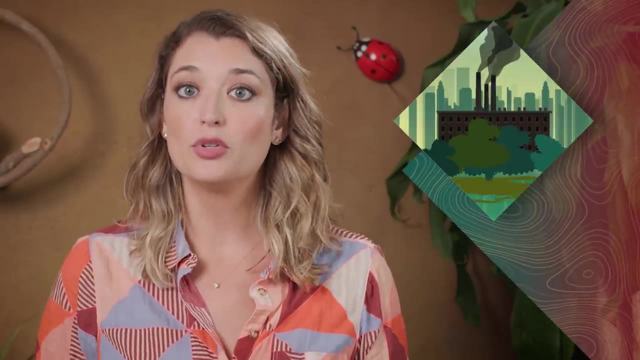 Urban areas are also centers of diffusion and cultural exchange that can drive innovation and new economic frontiers and technological advances. But large concentrations of people also create pressure, Partly because of the same economies of scale that make it efficient to offer services like education and renewable energy. there's also a lot of waste, pollution and strain. 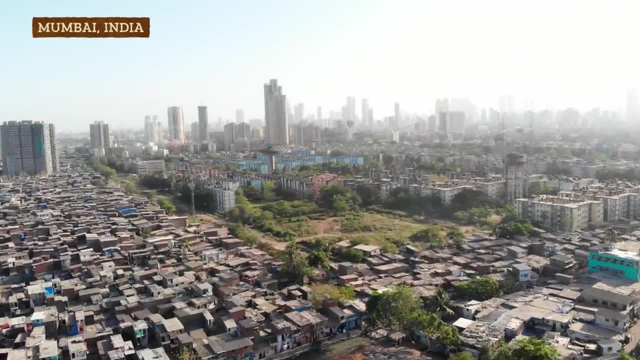 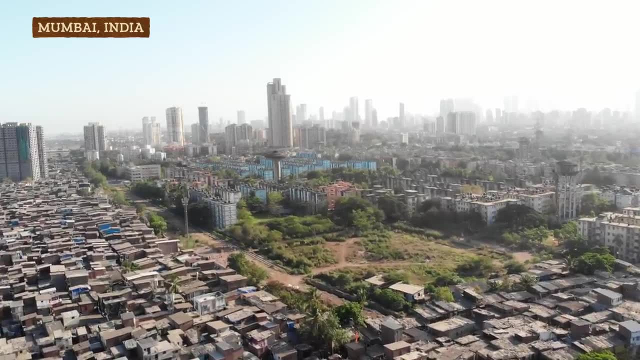 on water resources, And while there are more services in urban areas, they're not distributed evenly, Which can create uneven health outcomes. One strikingly visible example of this is the gray-green divide. On the usually wealthier side, houses are comfortably nestled among shady, tree-lined 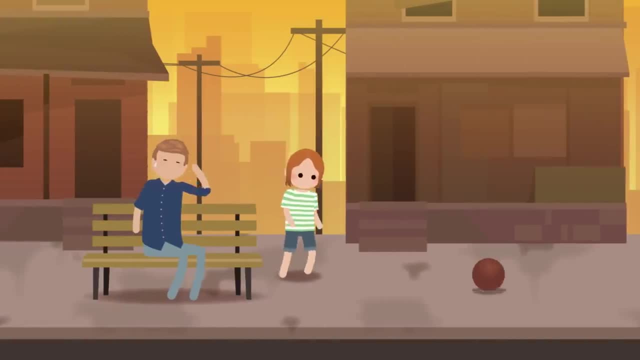 streets And on the other side of a single road, everything suddenly changes to shades of concrete and asphalt, Gray roads, gray roofs, gray sidewalks. This has an effect on our mood, our health and even the biodiversity of life around us. 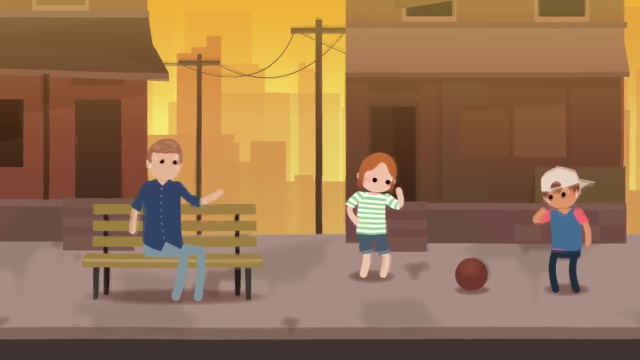 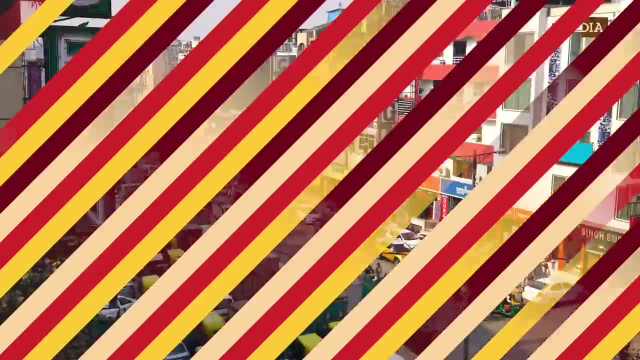 And all this vegetation also helps to minimize the effects of the urban heat island, Where all that asphalt, concrete, stone and steel absorbs heat and prevents air pollution from dissipating. In fact, whether air pollution is common because of the physical geography of the city or 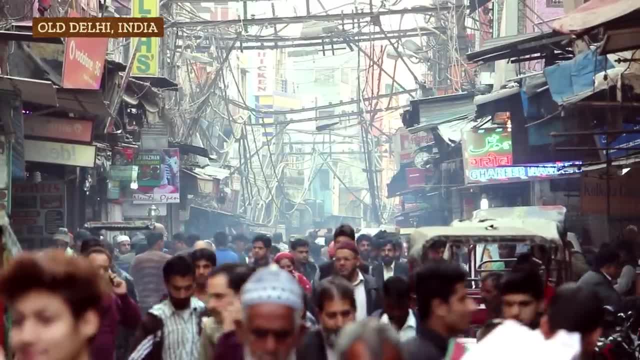 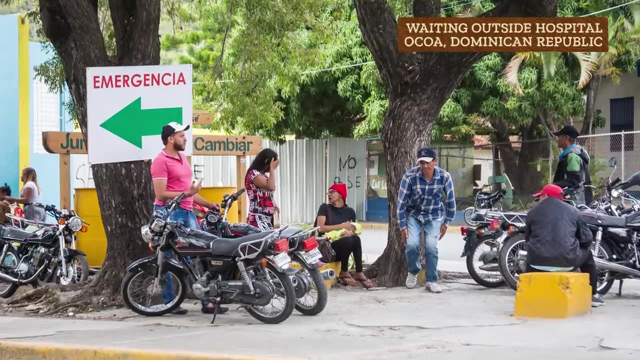 because there are more heavy polluters like cars or factories, there are a lot more asthma cases, ear-nose-throat illnesses and people with weaker immune systems in cities. This is particularly true in poorer areas of cities with substandard housing, where 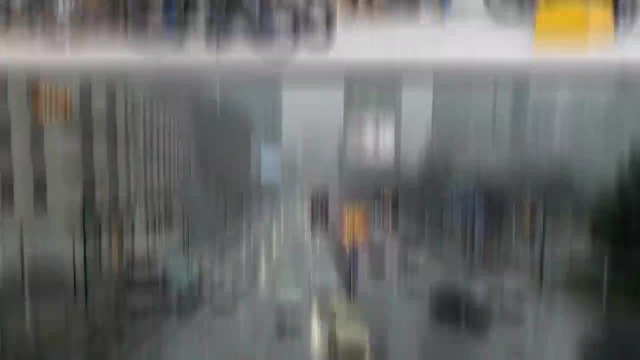 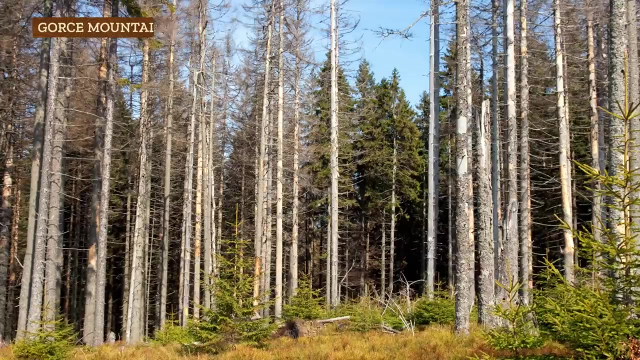 people have the fewest resources and little ability to access healthcare. There are other problems too, Like air pollution from factories. Air pollution from factories and cars can mix with water in the atmosphere, creating acid rain, The effects of which can be felt hundreds of miles away from the cities where it formed. 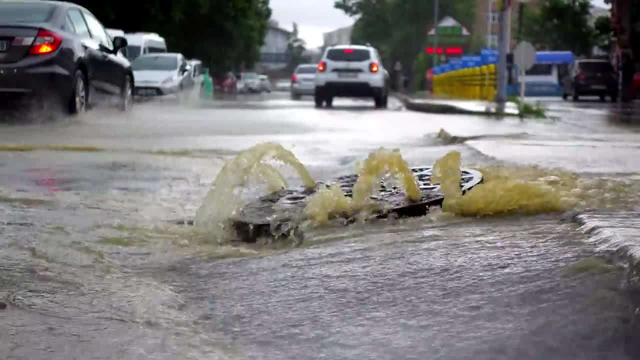 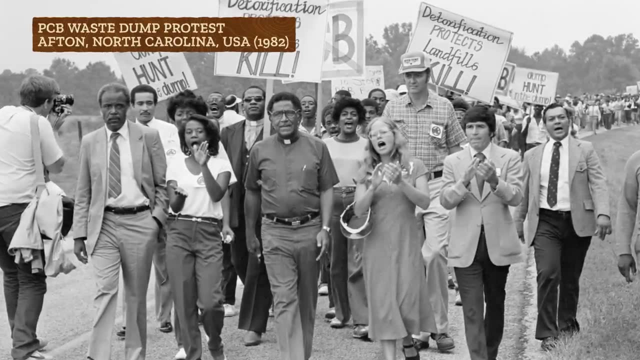 And there are water quality issues like sewer overflows and dumping chemicals in urban waterways. Most cities were built long before environmental justice was part of the urban planning discussion Which, according to the US Environmental Protection Agency, grew out of the civil rights movement. 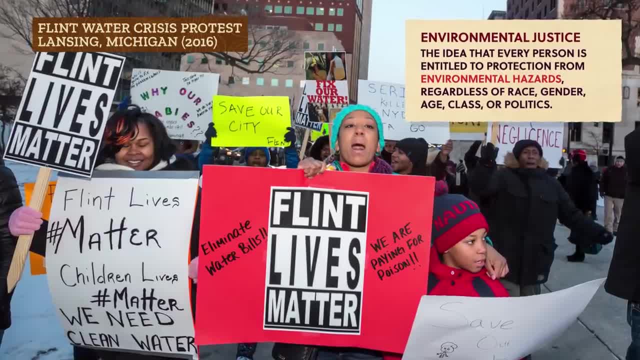 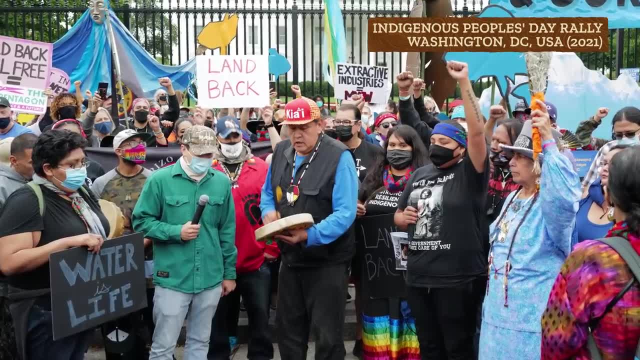 in the 1960s, and is the idea that every person is entitled to protection from environmental hazards, Regardless of race, gender, age, class or politics, And so creating sustainable cities is about planning for the future and reconciling the past, 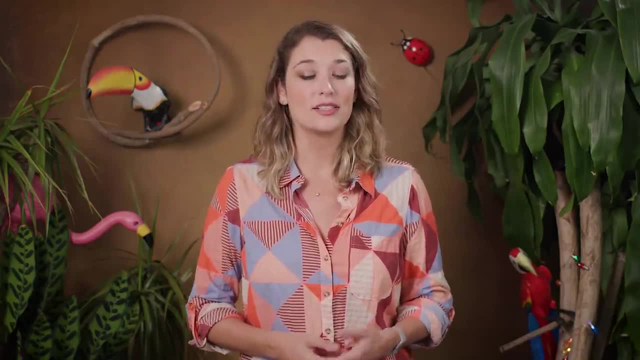 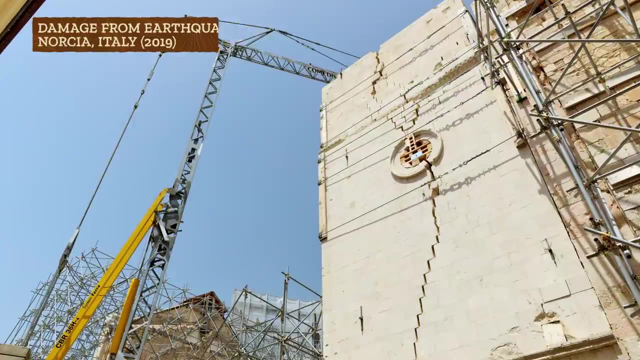 And as we work to make the built environment evolve with our own understandings of justice and environmental impact. there's a tension between retrofits that reuse old materials and spaces and fresh development. For instance, we have to decide what to do about beautiful old buildings built in areas. 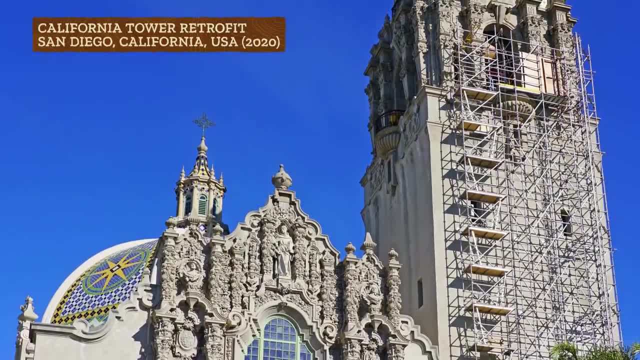 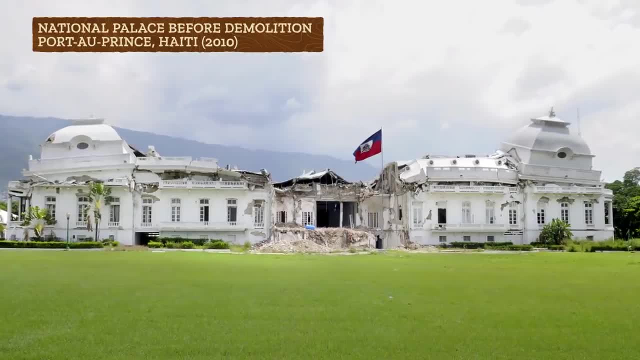 with lots of earthquakes. Urban planners may work with structural engineers to determine what kind of retrofitting is necessary to make a building earthquake-proof, or if the safest thing for everyone is to have the building come down And reusing what's there, like the work of French architects Anne Lacaton and Jean-Philippe. 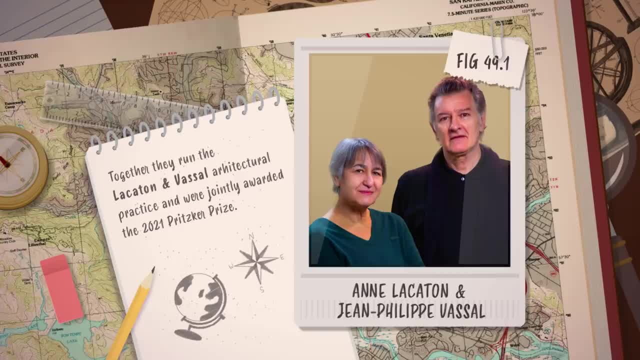 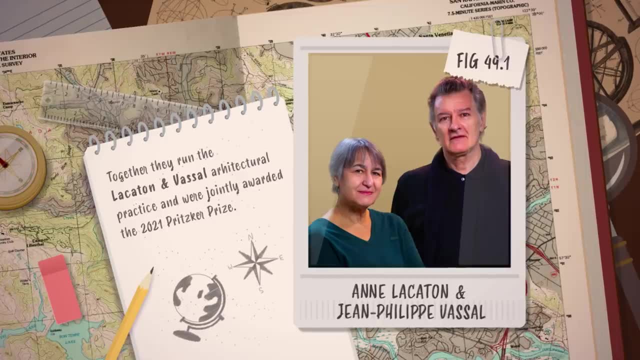 Vassal, who have won awards for their work. retrofitting buildings can have enormous global impact. The materials and construction industries are responsible for 10% of the world's greenhouse gas emissions in the early 2020s, which will be reduced dramatically if existing buildings. 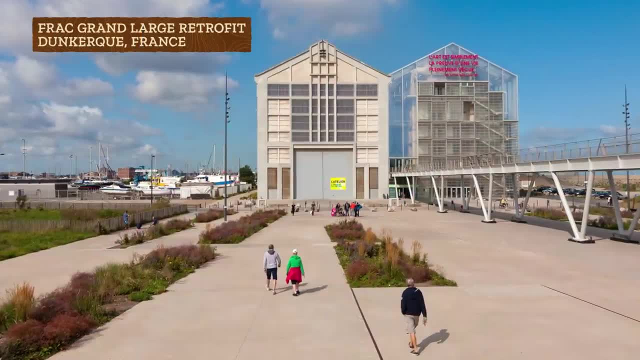 and infrastructure can be reused. The push to reuse rather than build fresh is a huge challenge, And it's not just the construction industry, It's also the infrastructure industry. It also saves biodiversity outside cities and minimizes how many habitats get fragmented. 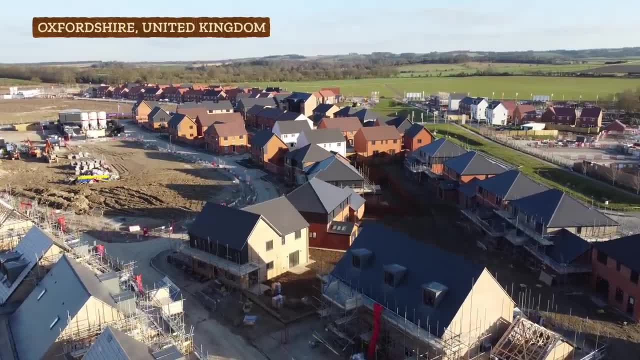 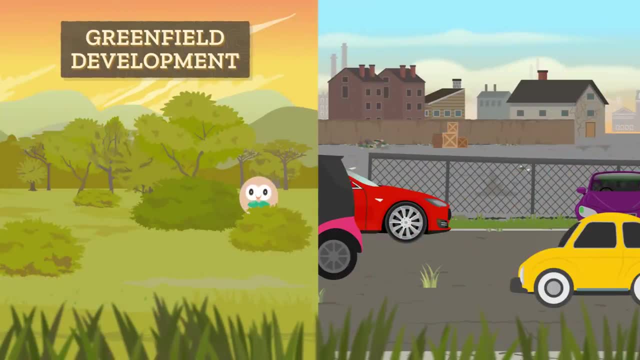 when urban sprawl is allowed to run amok. Much of this can be at risk when a greenfield development is chosen over a brownfield development. whether for housing, shops or factories In a greenfield development, the project is a blank slate for the architects and builders. 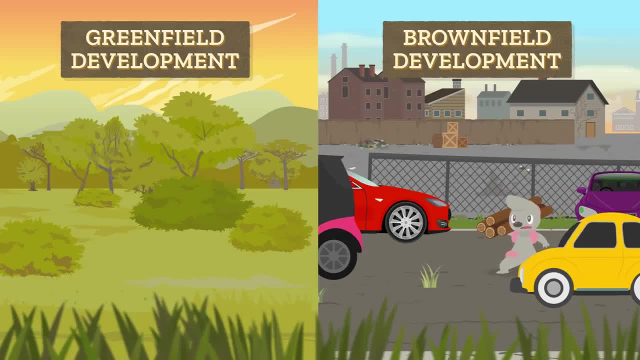 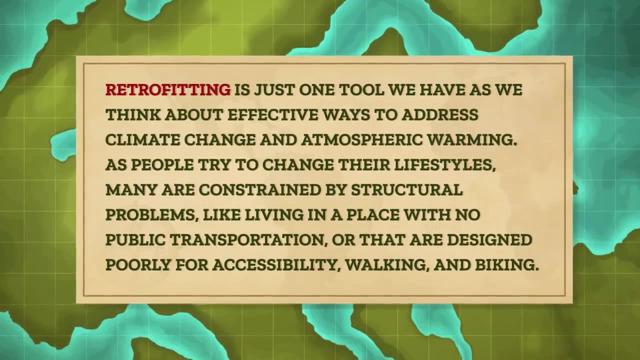 While brownfield development is done on top of land that has already been used, whether that land used to be a factory, car dealership or even a parking lot. Retrofitting is just one tool we have as we think about effective ways to address the 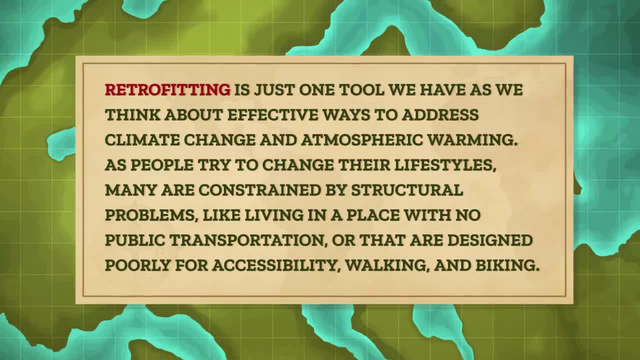 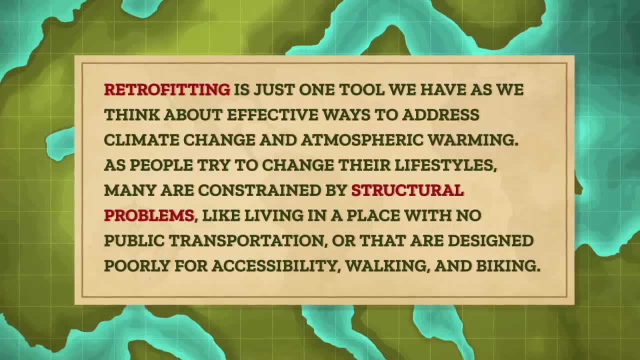 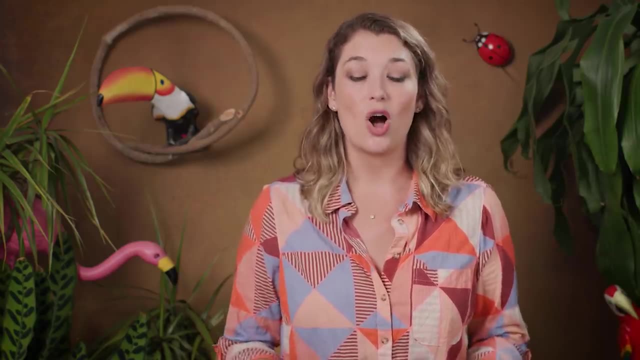 climate change and atmospheric warming. As people try to change their lifestyles, many are constrained by structural problems like living in a place with no public transportation or that are designed poorly for accessibility, walking and biking. Planning with an eye towards sustainability and working with what already has been built. 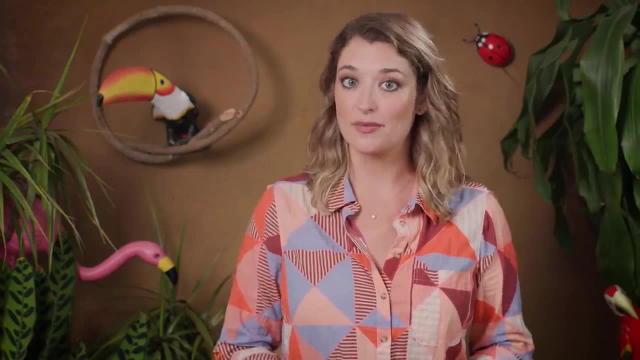 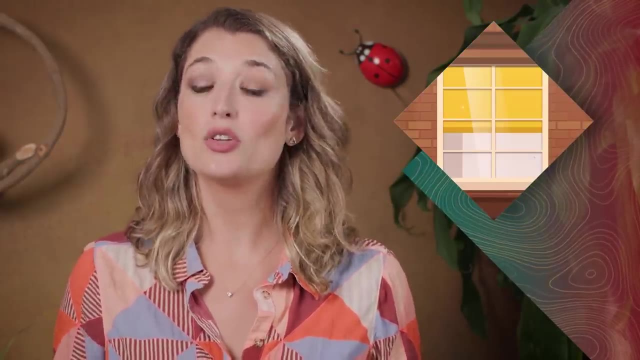 offers a way to start addressing those larger retrofits we need as a society And if we're going to shift to new technologies like electric cars, or retrofits like efficient windows and insulation, we have to also make space and be willing to have a space where 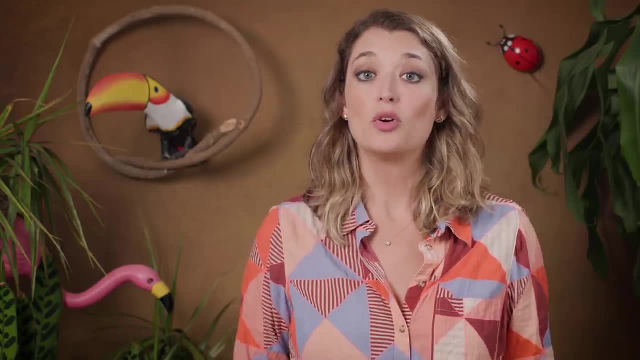 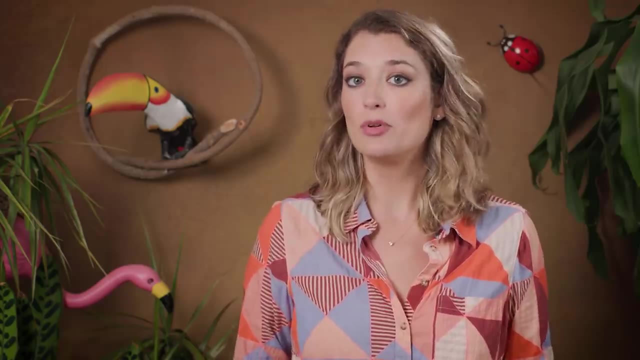 we're willing to help those who can't afford the changes. Who pays for retrofits or who pays the environmental costs for unsustainable designs are political. As a society, we often just accept that there will be some people who have to live with. 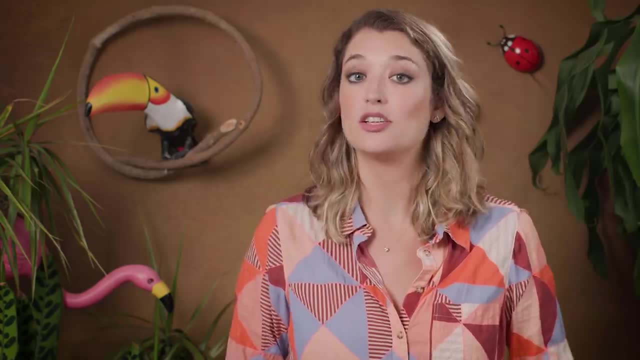 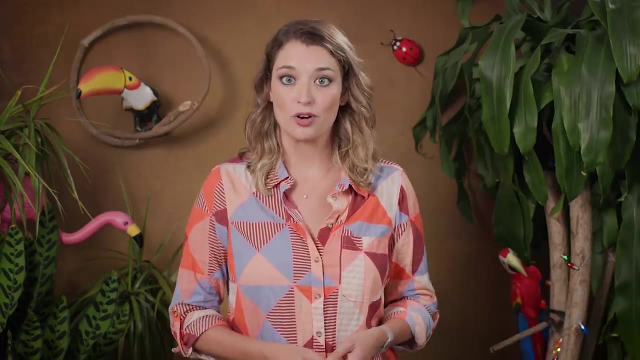 the economic or environmental consequences of the types of development decisions we make, And that can be heavily placed on vulnerable groups. So creating sustainable cities can't just be a part of our future, It also has to be part of our present, And that means citizens like you or I can get involved. 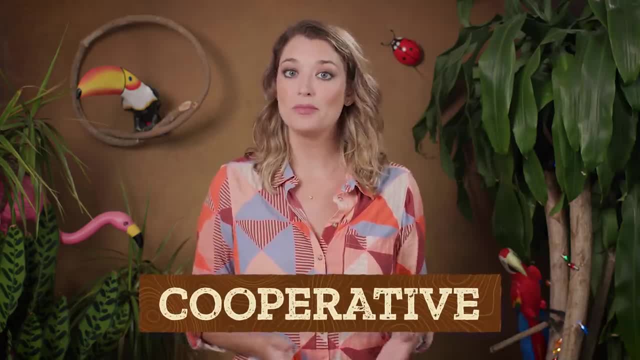 For example, a cooperative or co-op can be a part of our present, And that means citizens like you or I can get involved. For example, a cooperative or co-op is a group of people who come together to collectively manage a resource, whether that's housing or agricultural production. 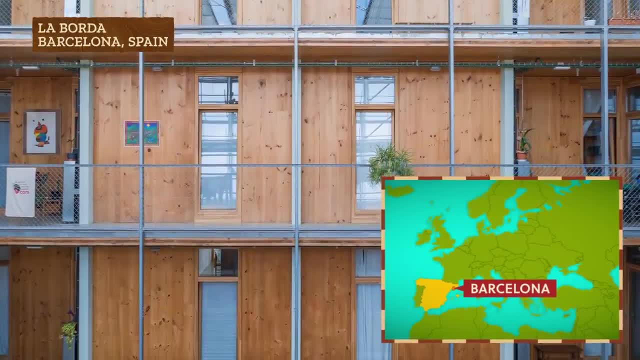 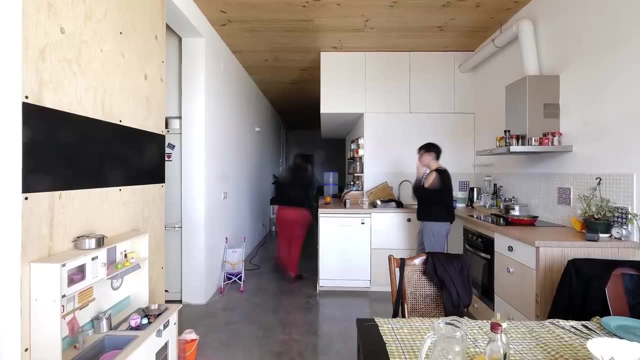 And in Barcelona, the Laborda Co-op is building off a collaborative housing model used in Denmark, Germany and Uruguay that provides non-speculative housing. This means that people don't own the individual units they live in, but they also don't pay. 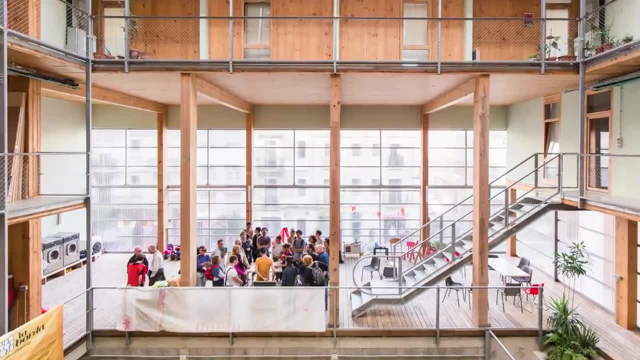 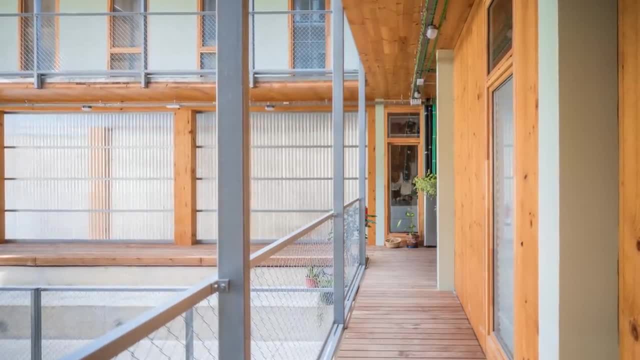 rent to another person or company. Instead, they join a cooperative business as members. It's a little complicated, but what's important here is that it's a way of opting out of trying to always make a profit on land or housing. Individuals can't sell or even rent their space in the co-op, and this keeps prices. 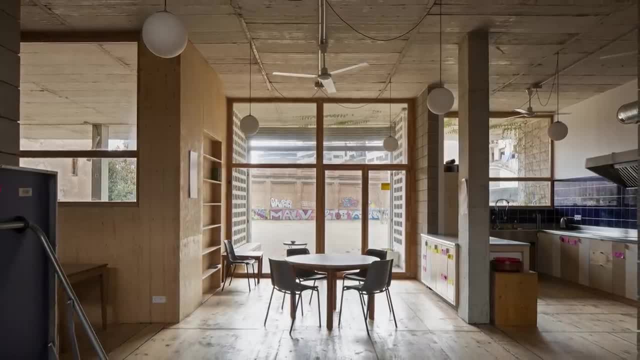 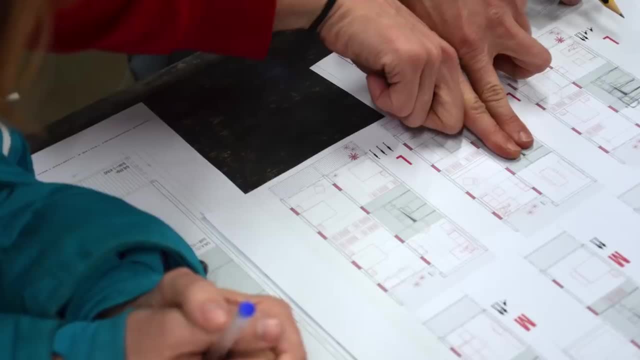 low for everyone. The complex was also built to be flexible in order to meet the needs of each of the residents. In fact, their building wasn't completely finished before people moved in. This allows the co-op members to finish the building to suit the needs of the group rather.